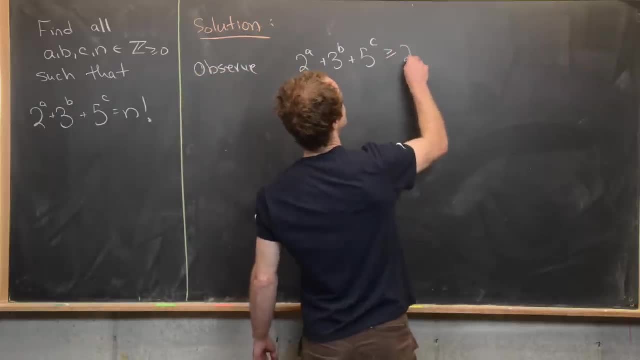 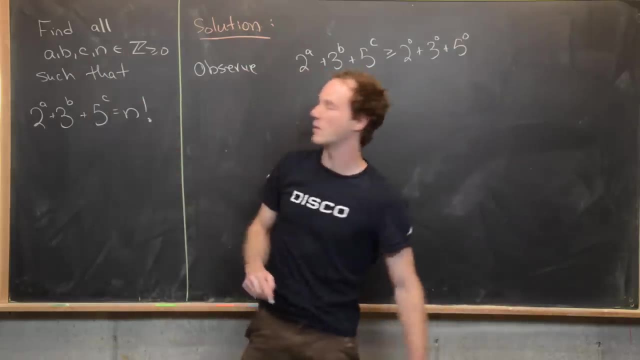 Which is always going to be bigger than or equal to 2 to the 0 plus 3 to the 0 plus 5 to the 0, given that a, b and c are always bigger than or equal to 0.. But notice, that's going to be equal to. 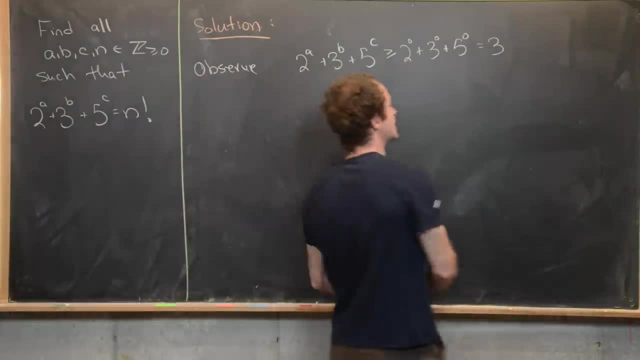 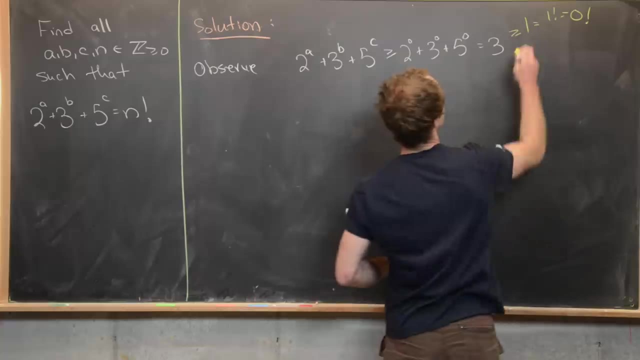 3. But now notice that 3 is bigger than 1, which is equal to 1 factorial, which is equal to 0 factorial, And 3 is also going to be equal to n factorial, And so what we're going to do is we're. 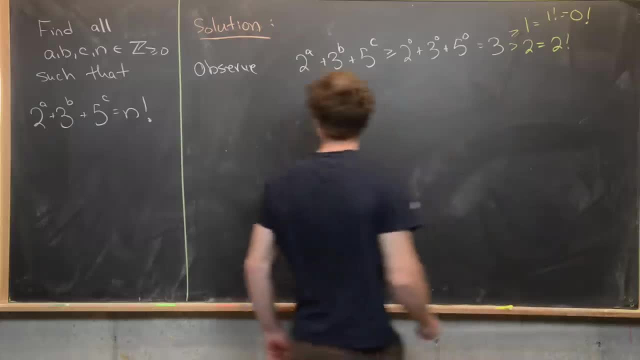 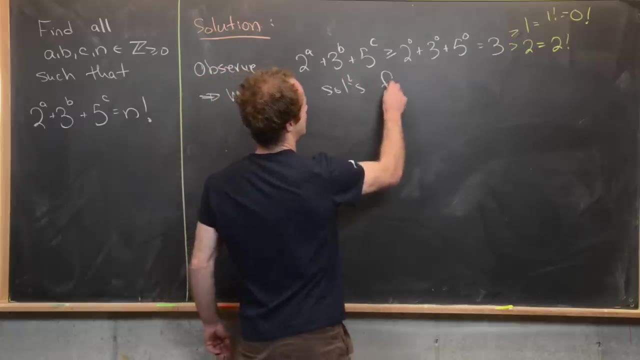 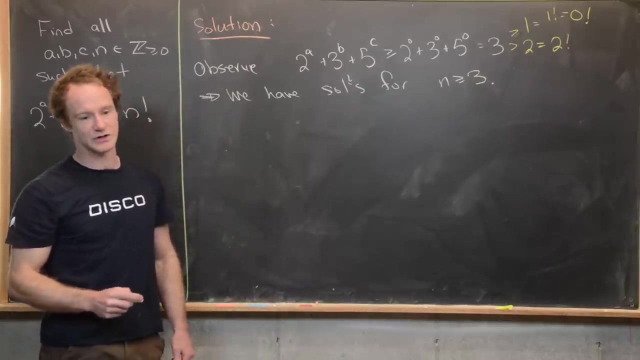 bigger than 2, which is equal to 2 factorial. So that immediately tells us that we only have solutions for n bigger than or equal to 3.. So we can't have n equal 1 or n equal 2.. So that's a good place to start, and now we'll start. 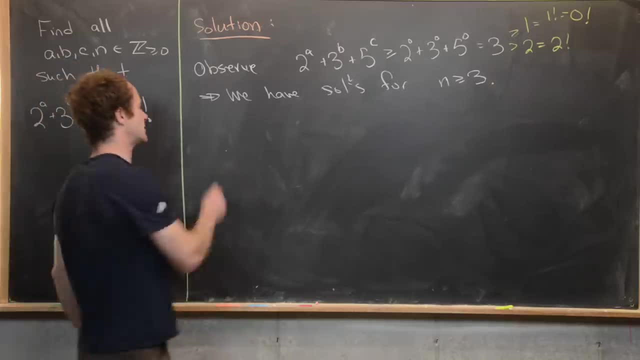 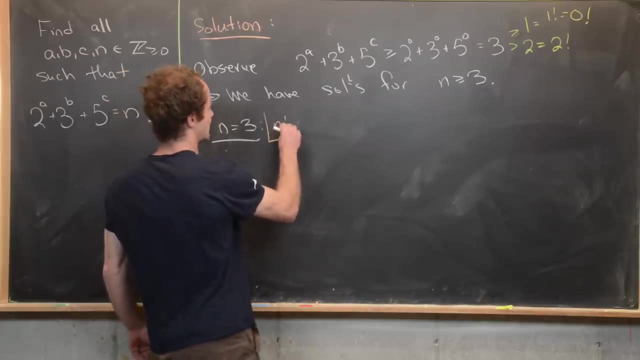 looking for some of these small solutions. So we'll look at our first case, maybe when n equals 3.. So notice, when n equals 3, that's the same thing as saying n factorial equals 6.. So we're looking for solutions when some power of 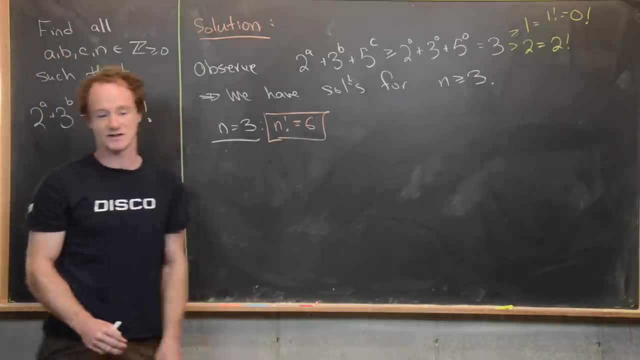 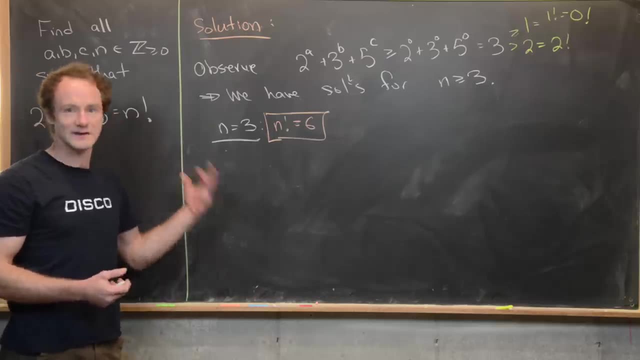 2 plus some power of 3 plus some power of 5 equals 6.. So we've got to just play around with it, find a couple and then argue that there are no more, before moving on to n equals 4, and so on and so forth. So the first thing that I want to 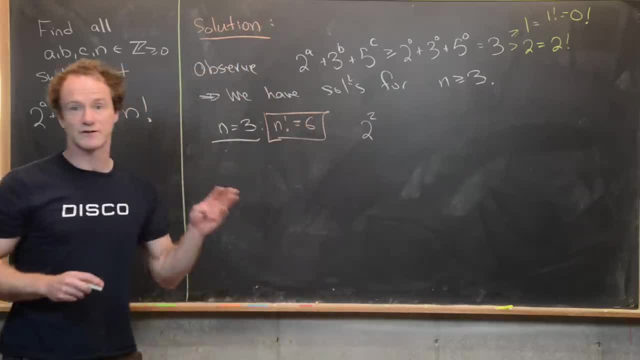 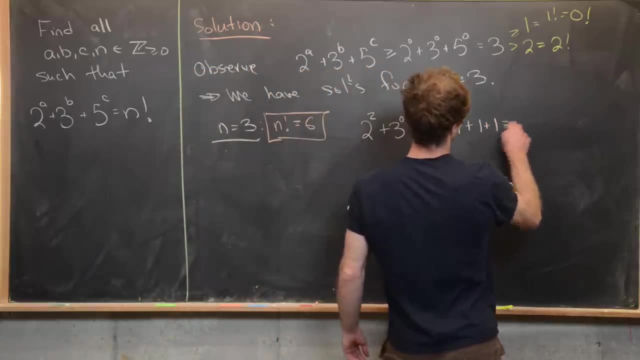 notice is: if we take 2 to the 2, that's going to be equal to 4. and then if we add 3 to the 0 and 5 to the 0, we get 4 plus 1 plus 1, but that's equal to 6, but that's equal to 3 factorial. so we have 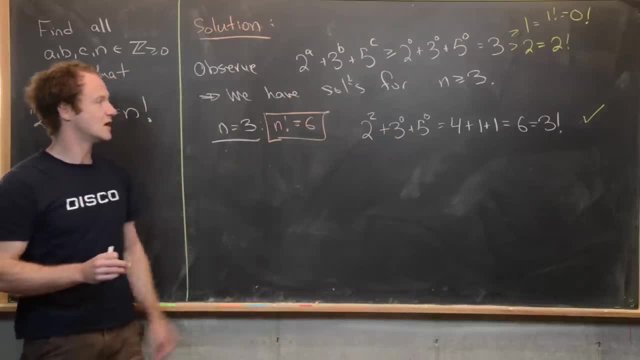 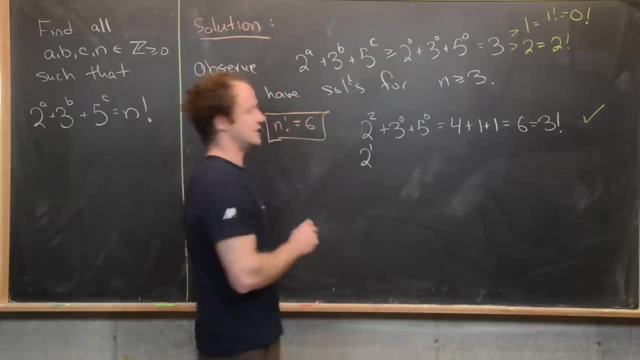 found our first solution, And then we can look at this just a little bit longer and we see that we have another solution, and so we can have a solution 2 to the 1, so that's going to be equal to 2 plus 3 to the 1 plus 5 to the 0. so notice. 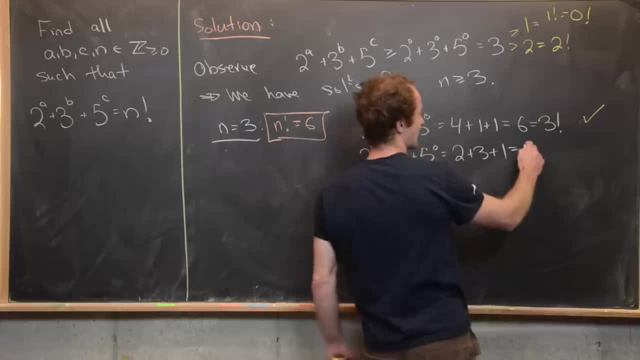 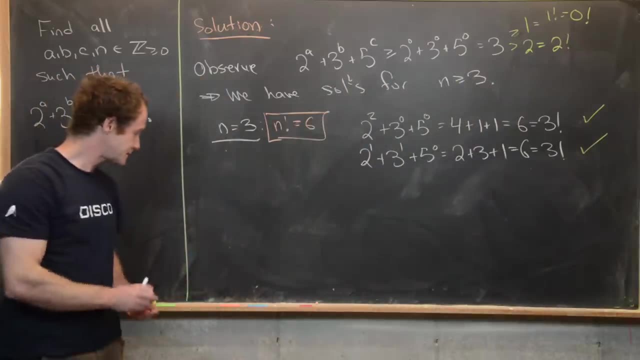 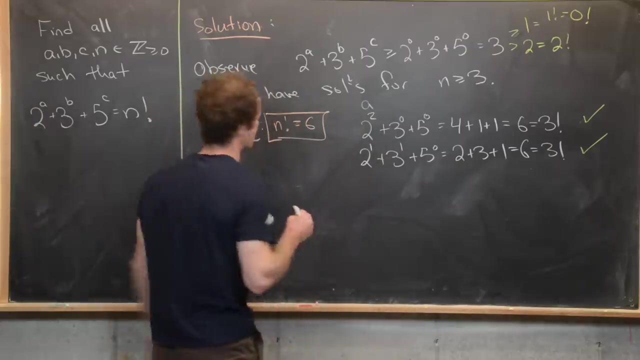 that is 2 plus three plus one, but that's gonna be five plus one, which is six, which is also three factorial. So again we've got another solution there, And now we can maybe easily argue here that a, in other words the power of two, 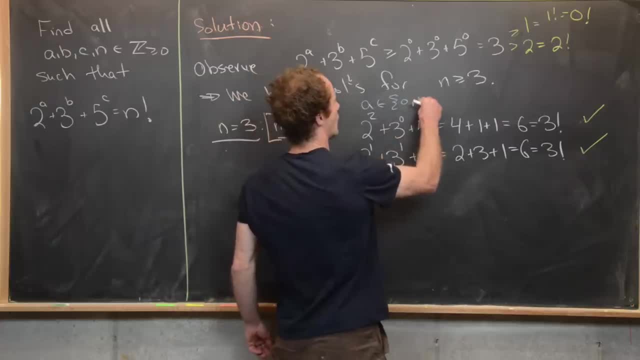 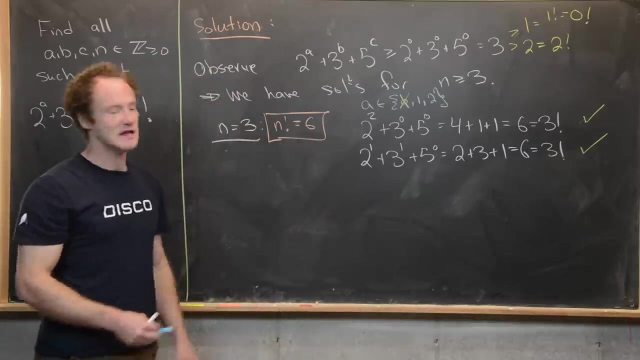 must be equal to zero, one or two in this case. And we know that it cannot be equal to zero, because if it were equal to zero, then the left-hand side would be odd, whereas the right-hand side would be even. So, the only possible values for a are one and two. 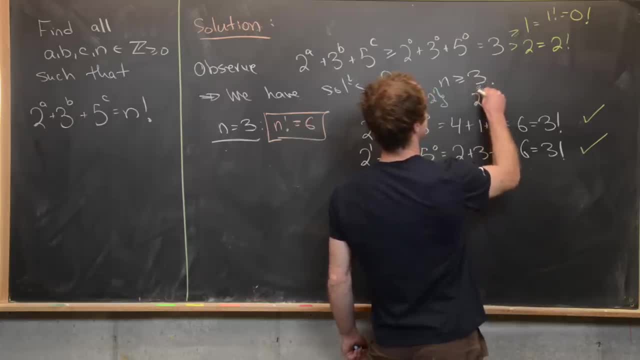 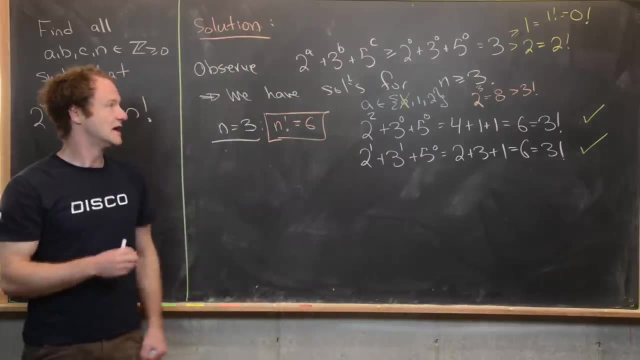 And I might wanna point out that's because we have two to the three is equal to eight, which is bigger than three- factorial Good. so we can't even get started if that a is bigger than three. And so now we've got solutions for a equals one and two. 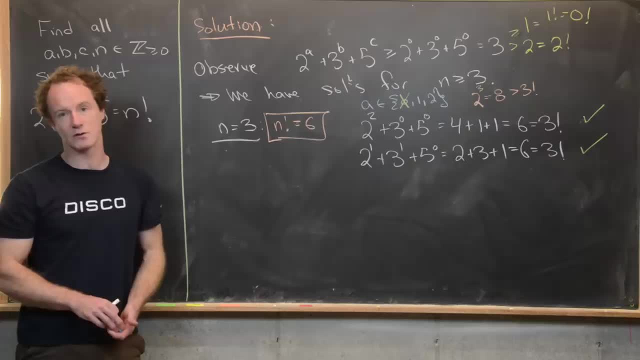 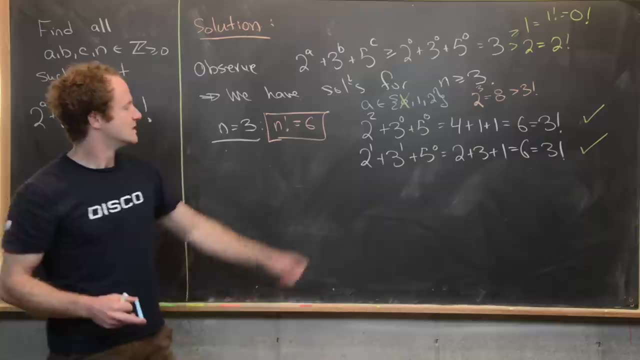 and now we just have to argue that those are the only solutions when a equals one and two. So I'll let you guys maybe think about that, but you can do something similar to what we did here. So notice here the only possibility for b and c. 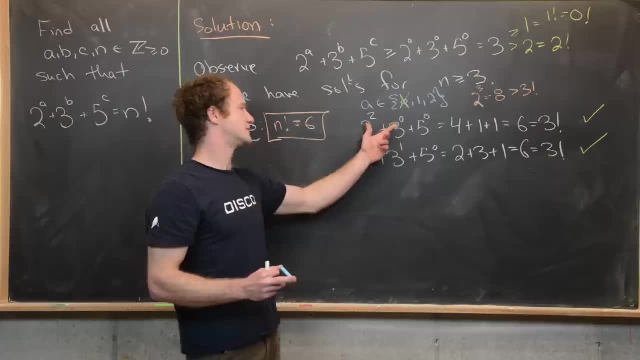 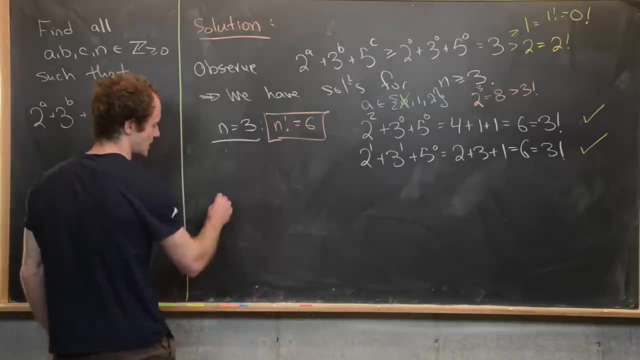 are both zero, because immediately we take something larger and we're bigger than six, and then something similar happens down here in this equation as well. Okay, so now let's go on to our next case, which is when n equals four and when n equals four. 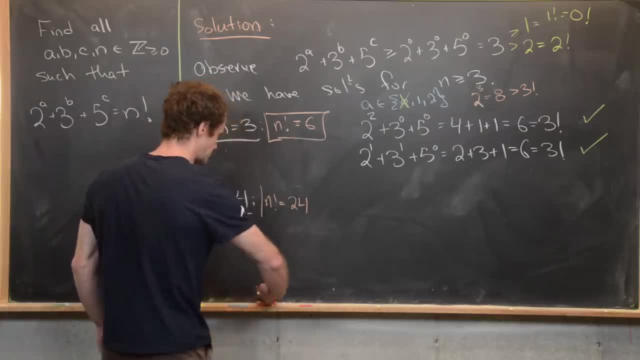 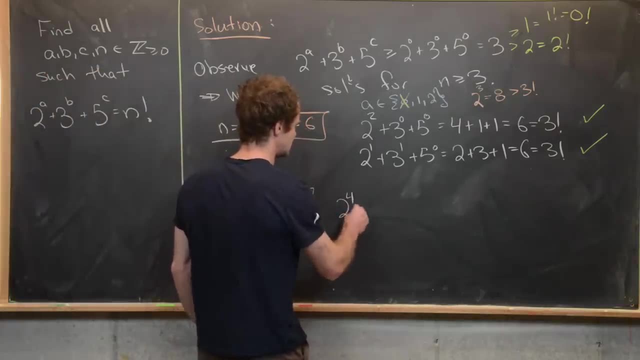 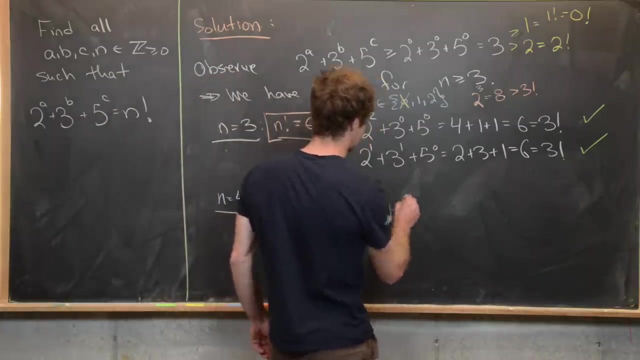 n factorial. N factorial is equal to 24,. good, And there's one solution in this case as well, and that's gonna go like this. So it's gonna be two to the four, so that's 16, plus three to the one, plus five to the one. 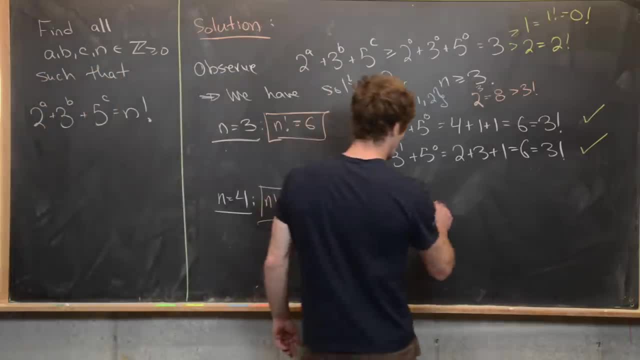 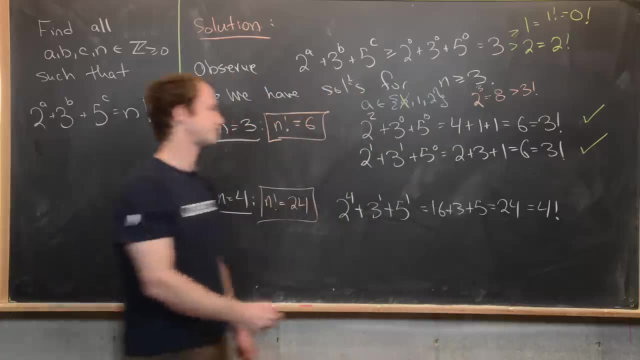 so it's 16 plus eight, In other words 16 plus three plus five, which is equal to 24, which, like I said, is four factorial. Then we can make a similar argument: that we have no more solutions to this equation either. 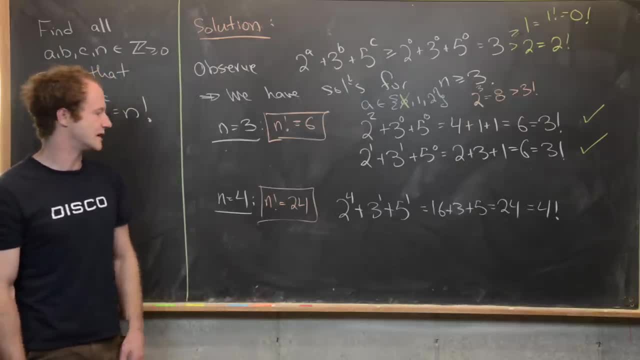 Notice, if we have two to the five, that's 32, that's already too big. But then if we look for smaller powers of two, those won't work either. just checking case by case. Okay, so we've got three solutions. 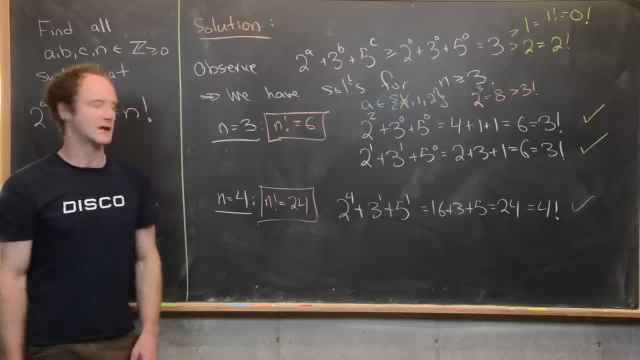 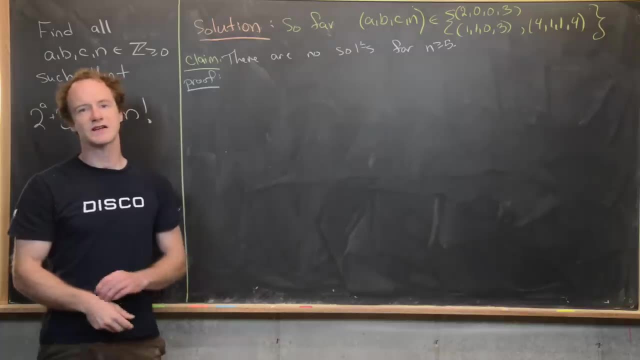 We've got two solutions where we get three factorial and one where we get four factorial. Now maybe I'll go ahead and clean this up and I'll show that these are actually the only solution. So we just got done arguing that we have three solutions. 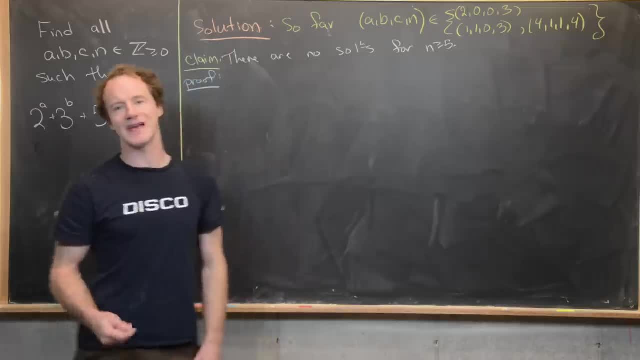 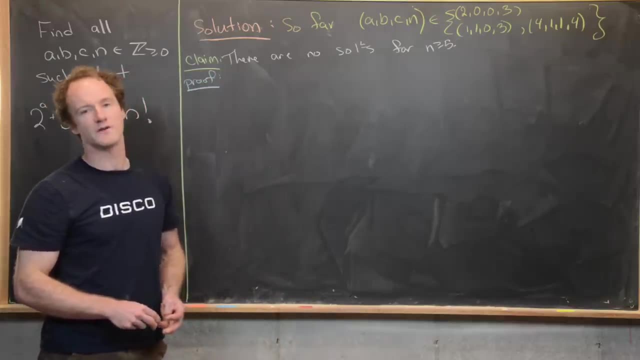 for n equals three and four, and those are given by the quadruples a, b, c, n is two zero, zero three. one one zero three or four one one, four. Now we wanna prove the following claim: 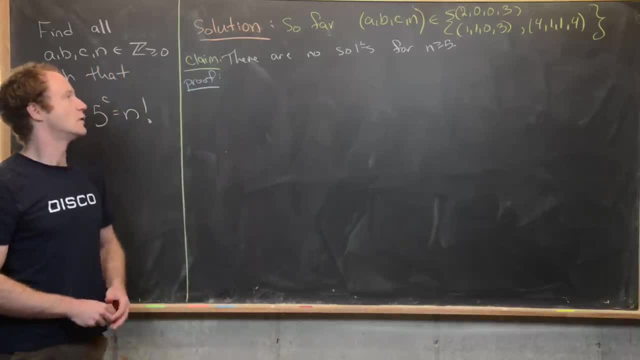 which will finish off the whole problem, and that is, we wanna show that there are no solutions for n bigger than or equal to five, and we're gonna do this by working modulo five factorial, in other words modulo 120.. Maybe first, 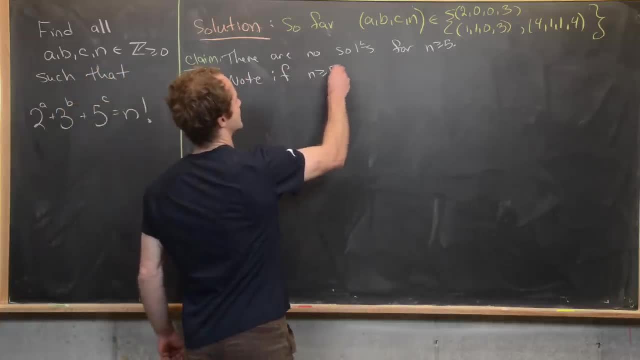 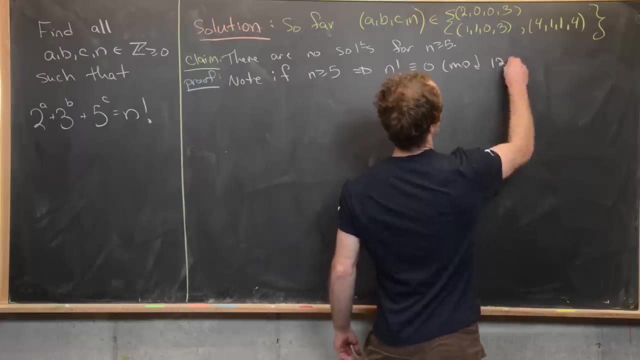 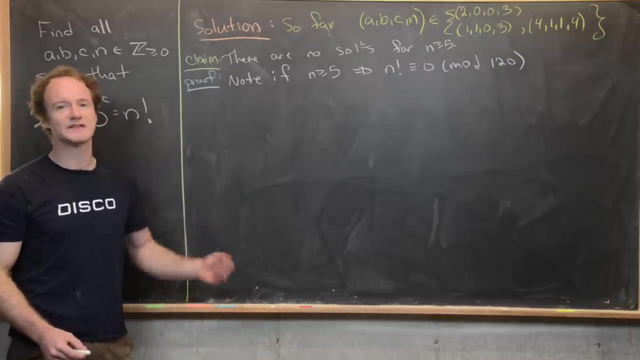 we'll go ahead and notice that if n is bigger than or equal to five, then that means that n factorial is congruent to zero mod five factorial, which is 120.. It's because, like, six factorial is gonna be a multiple of five factorial, and so on and so forth. 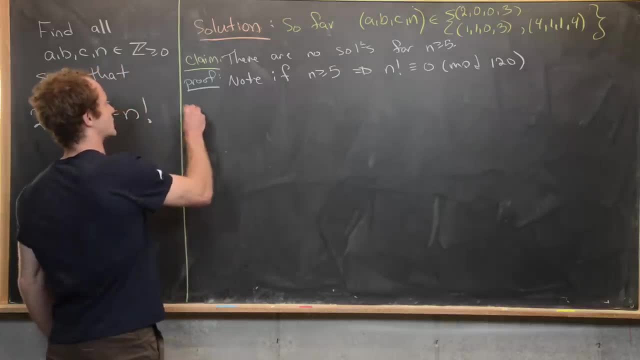 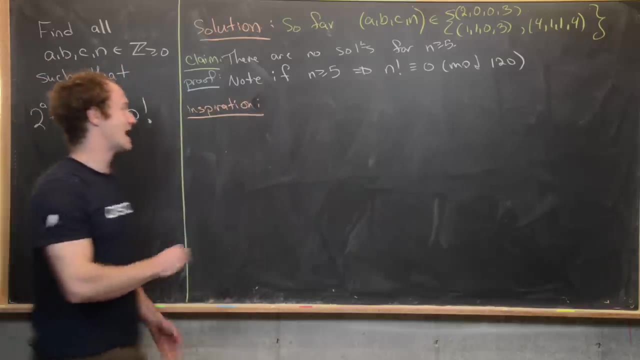 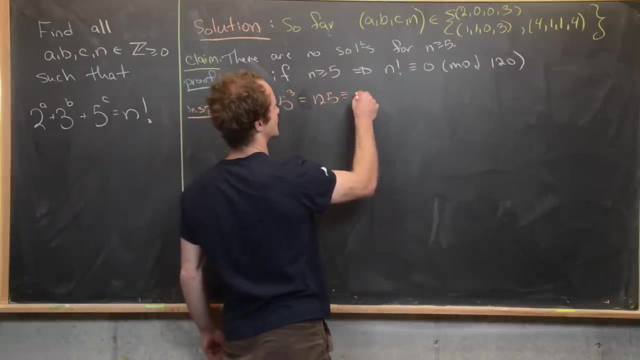 Good, and now we want to take the following inspiration as a reason for making the following next step, and that is: notice that if we take five cubed we get 125, but 125 is congruent to five mod 120.. 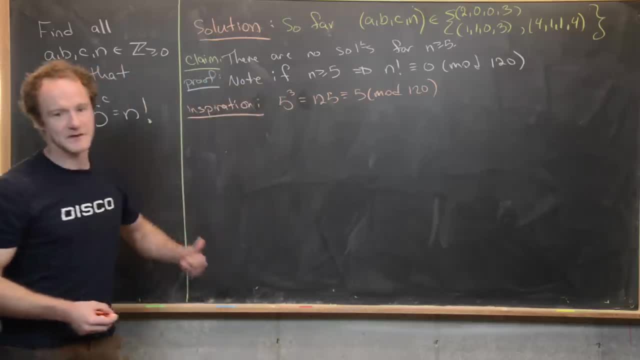 Notice that. that tells us that if we look at the powers of five mod 120, we only get three possibilities. We get one. so that would be like five to the zero: we get five and we get 25, but if we cube it, 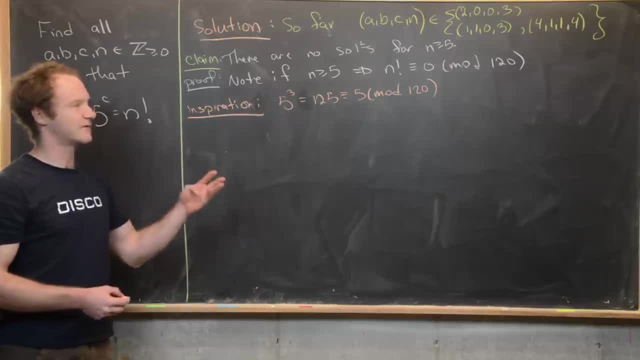 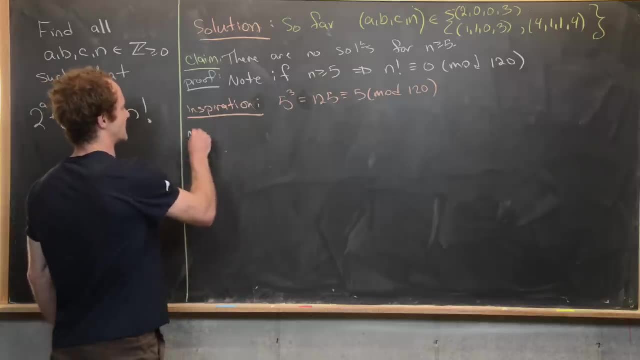 we get 125.. We get 25,, which is back to five, which means if we take the fourth power, we're back to 25, and so on and so forth. So maybe we could put all of this together with the following observation: maybe. 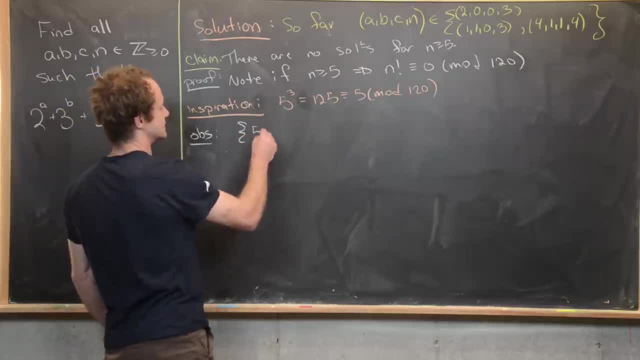 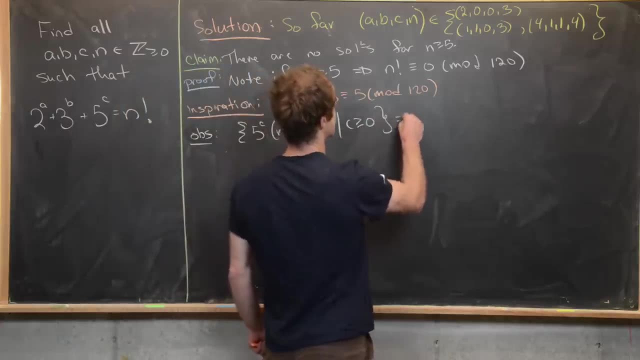 and that is if we look at all of the residues of five to the C mod 120, as C runs bigger than or equal to zero, we're only gonna get three numbers, and those numbers will be one, five or 20.. 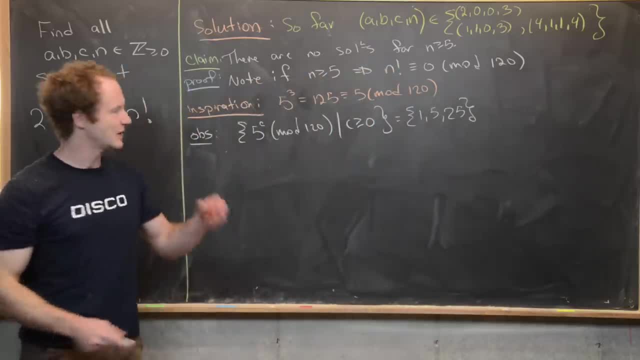 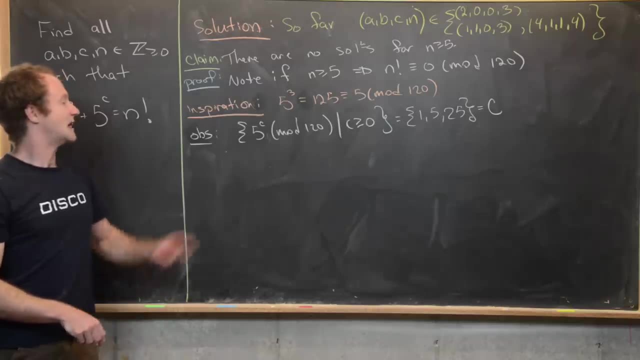 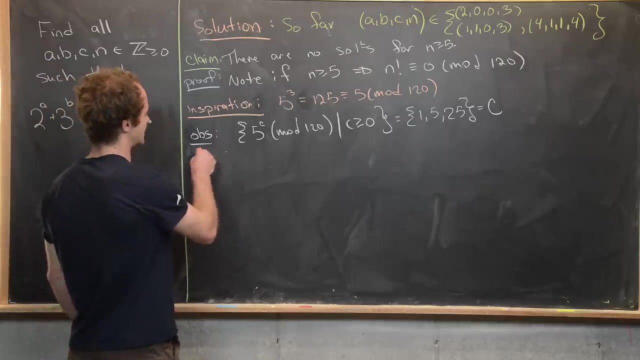 Five or 25, great, I'm gonna go ahead and call that set capital C, kind of to be in line of this little C right here. Now we can look at a similar structure within the powers of two and the powers of three. So let's go ahead and do that. 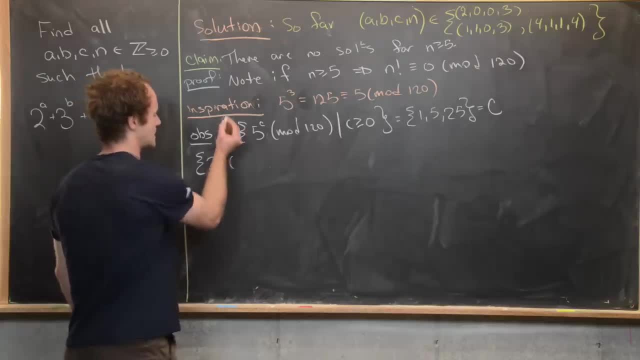 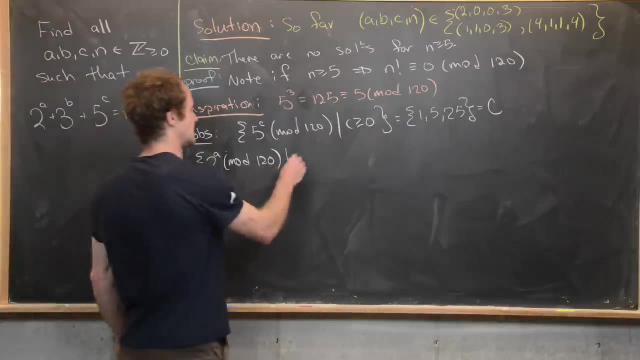 So for the powers of two, maybe I'll write that as two to the A mod 120, in other words the residues modulo 120 of the powers of two, and here we're gonna let A run one, five or 20.. 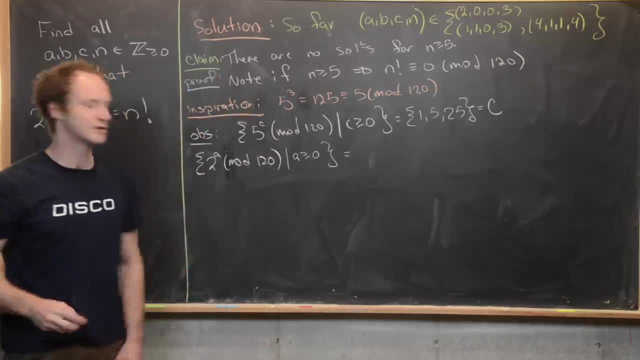 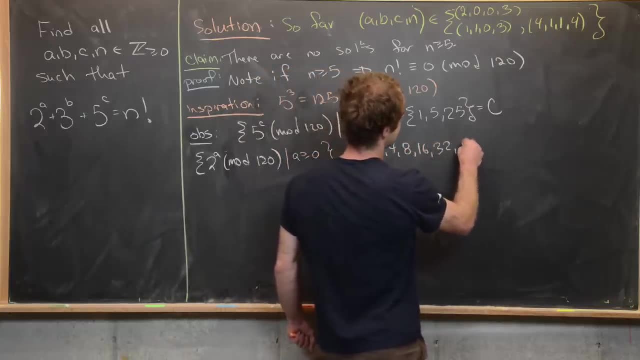 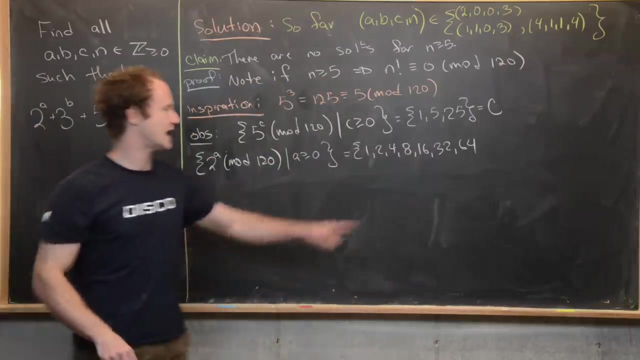 A run bigger than or equal to zero. So notice that this is going to be equal to one, two, four, eight, 16,, 32,, 64.. But now the next power of two is 128, but 128 is eight mod 120, so we're actually done. 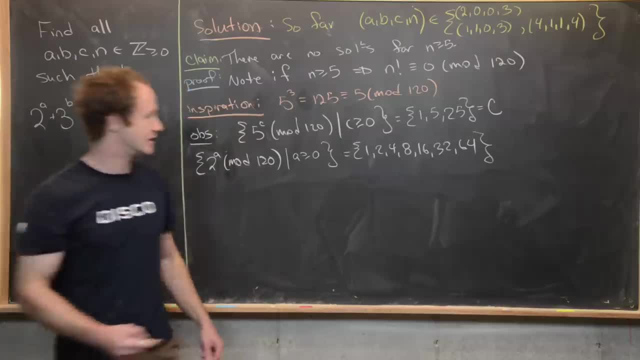 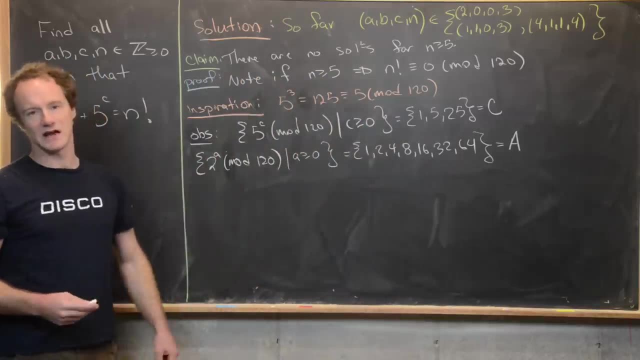 This is as large as the set needs to be. Okay, good, And I'm gonna go ahead and call this set A, A mod 120,, in other words, this set A mod 120, and I'm gonna leave it here. 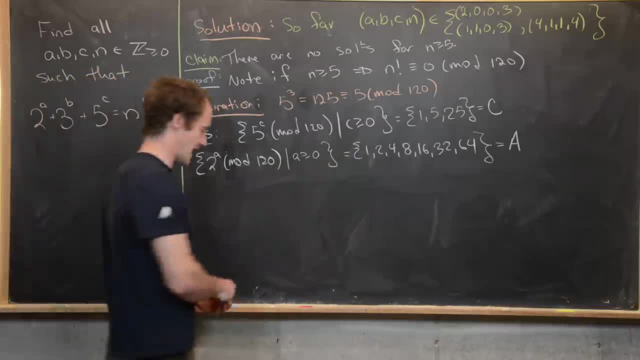 and I'm gonna call this set A mod 120, and I'm gonna move this to the right. I'm gonna use the number one symbol, I'm gonna make sure that I brought this one out and then I'm gonna leave that out. 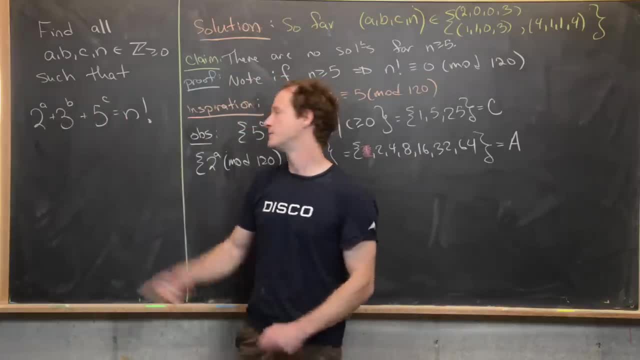 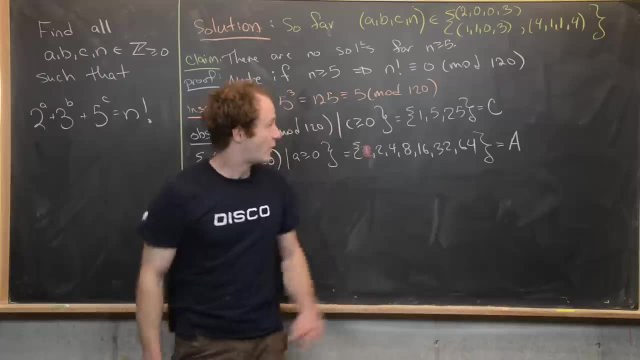 so that I can keep this one out, and that's gonna make this set A mod 120. So this is gonna be equal to number one in here. All right, so let's quickly go ahead and do the matrix ref and enter that right here. 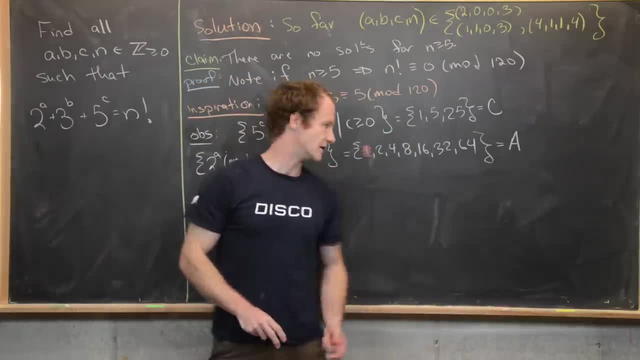 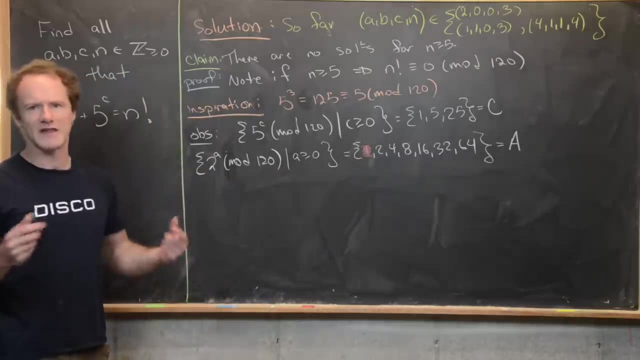 and look at the number one symbol and look at the number two symbol and look at the number two to be even. but all powers of two are even, except for two to the zero. so we can get rid of that one, because that will not produce a solution by that kind of simple parity argument. now let's go ahead. 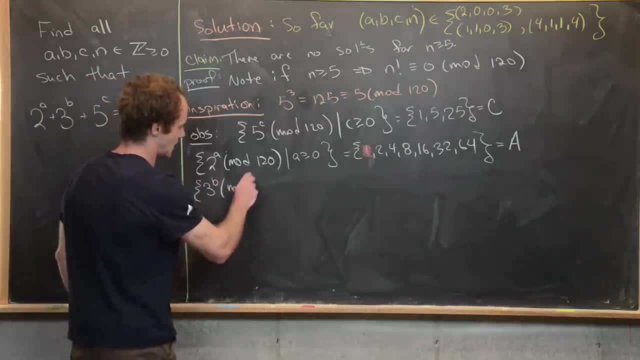 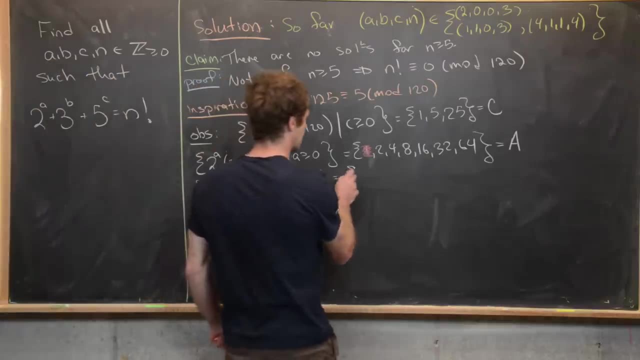 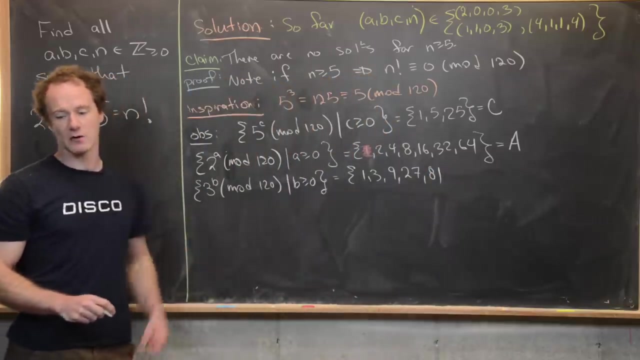 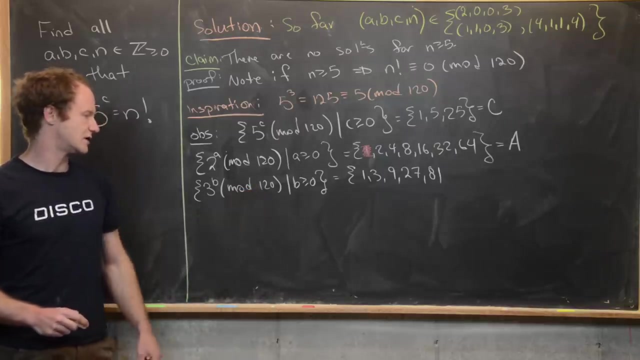 and look at this. so three to the b mod, 120 for non-negative integers b. so here we're going to get 1, 3, 9, 27, 81. then the next power of 3 is 243. but notice, 243 is 3 more than 240. 240 is twice 120. so 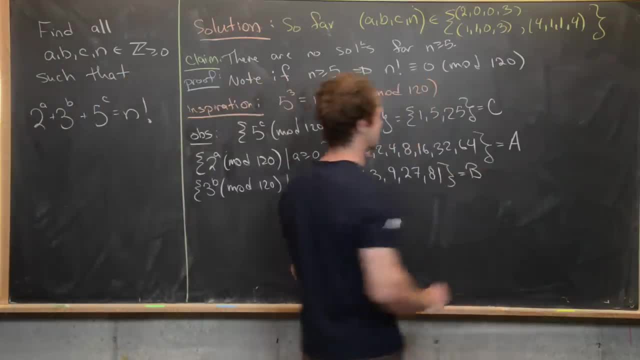 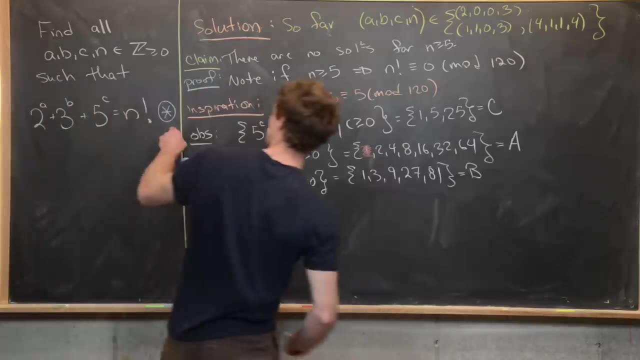 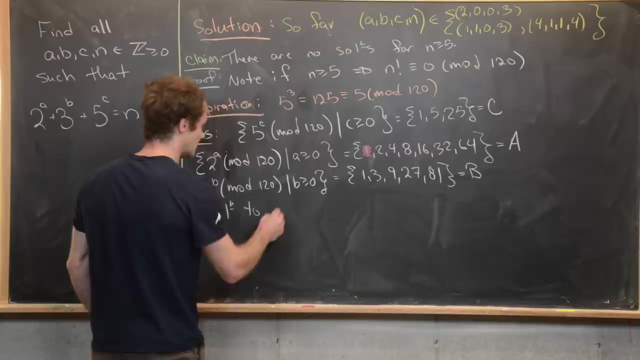 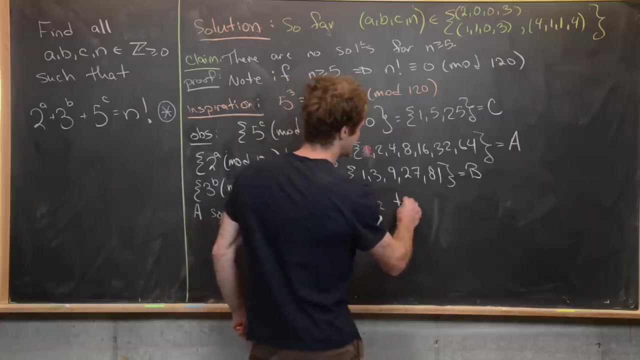 that means we can stop here and i'll go ahead and write this as b. good now. the next thing that i want to notice is that if i let this equation be star, a solution to this equation is going to be b. so a solution to star- maybe blue star- will give rise to a solution to the following: x plus y plus. 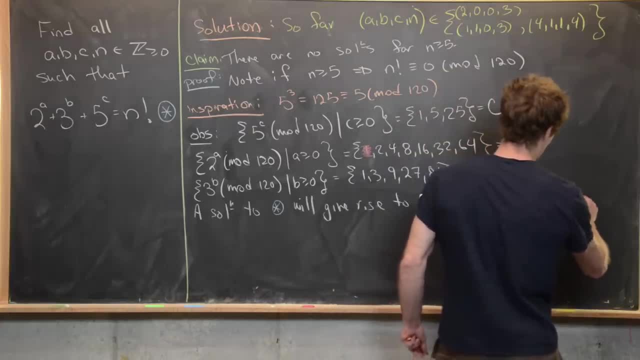 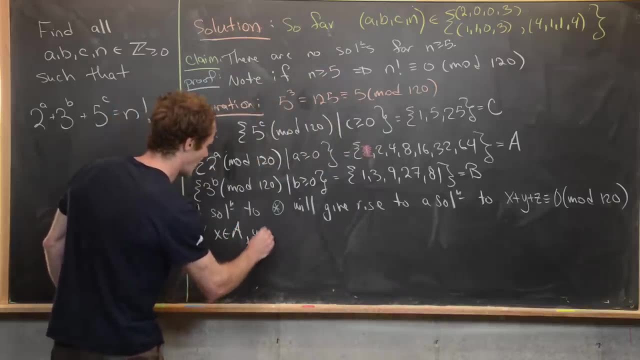 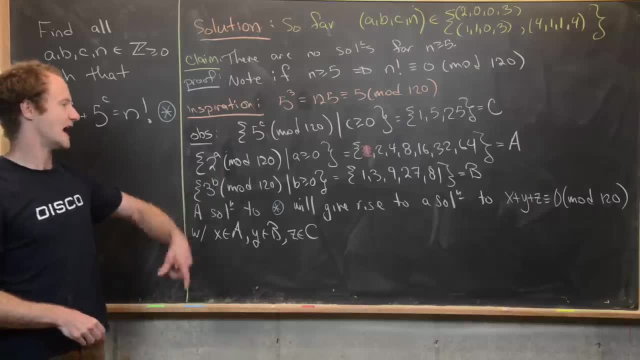 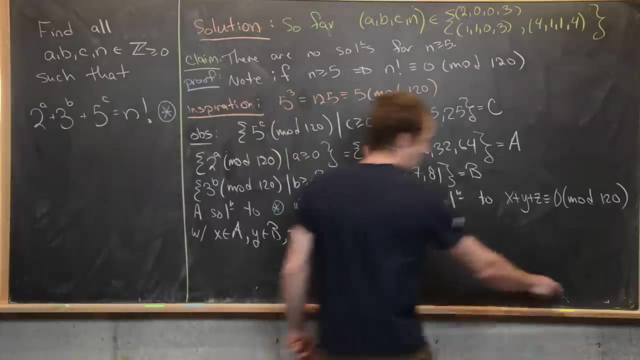 and z is in c. i should say that's because x is going to be a power of two, y is going to be a power of three and z is going to be a power of five. good, but notice that's going to give us six possible solutions to the following equivalent congruence. notice that this is equivalent to x. 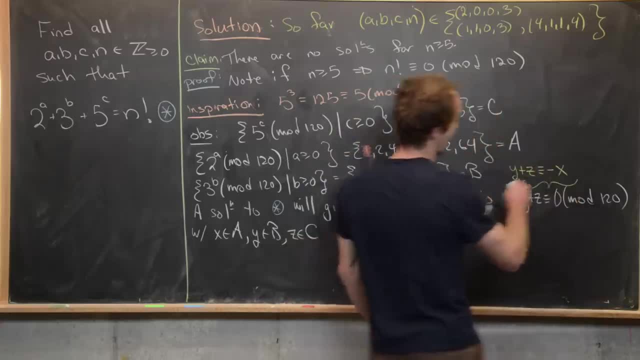 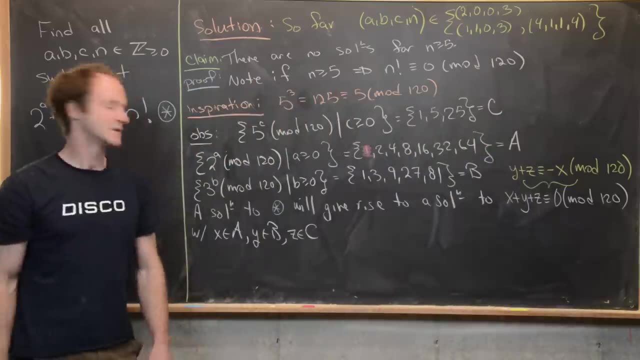 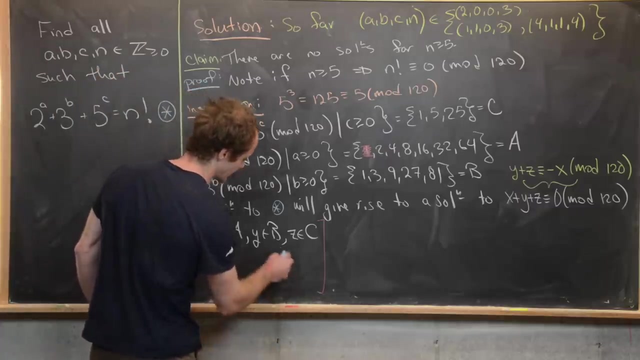 plus y is congruent to sorry y plus z is congruent to negative x. x mod 120.. good, so, like i said, this is going to give rise to a solution to the following, so a solution to one of. so, let's see, x, sorry y plus z is congruent to. now we just have to run through. 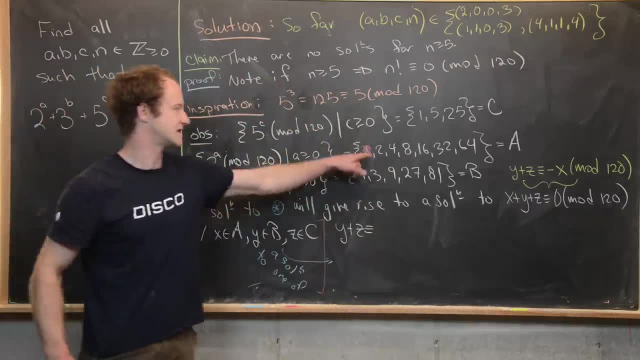 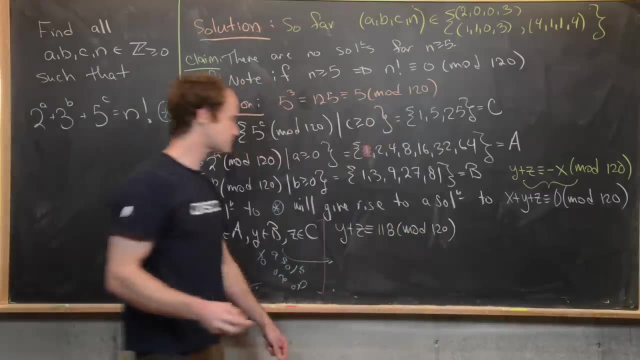 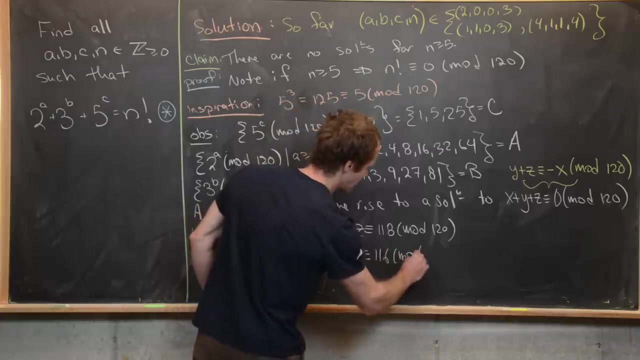 all values of negative x mod 120, where x is coming from this set. so negative 2 is going to be 118 mod 120. then y plus z congruent to. let's see that one's going to be 116 mod 120. then let's see what this one's going to be. that's going to be 112. so y plus z. 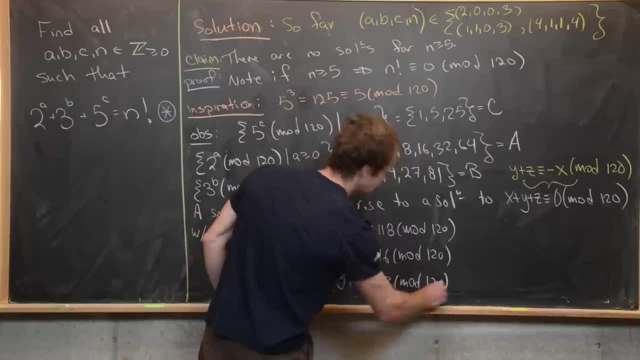 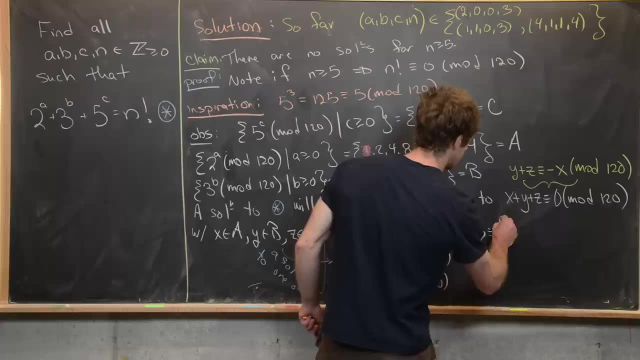 is congruent to 112 mod 120. then let's see the rest of them. so let's see this: 16 right here that's going to be: y plus z is congruent to 112.. 104 mod 120. the next y plus z is congruent to 88 mod 120, and then finally, y plus z. 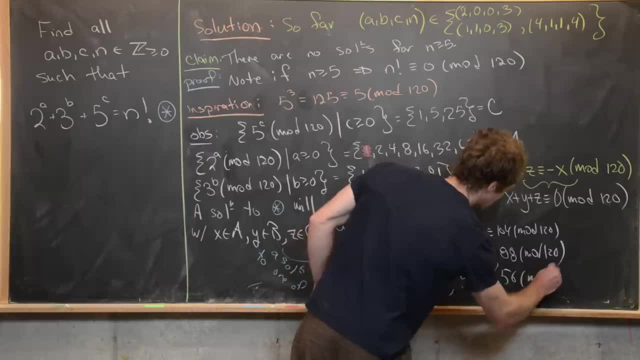 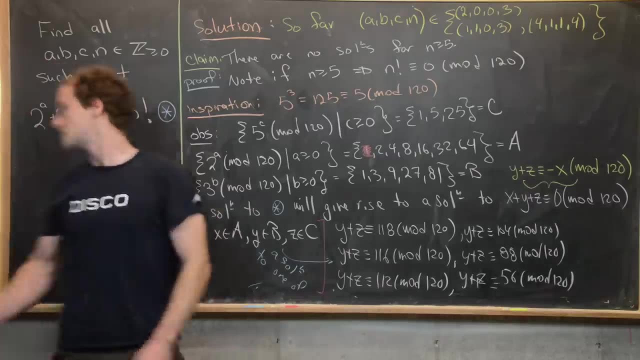 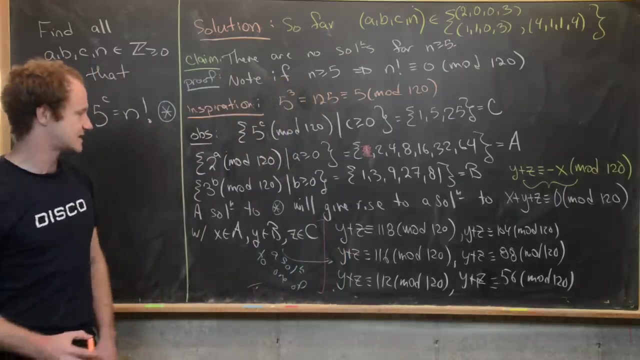 is congruent to 56 mod 120.. okay, so let's just like look at what we've done so far here. so if we have a solution to this equation, when n is bigger than or equal to five, then that's going to give us a solution to this congruence. x plus y plus z is congruent to 0 mod.